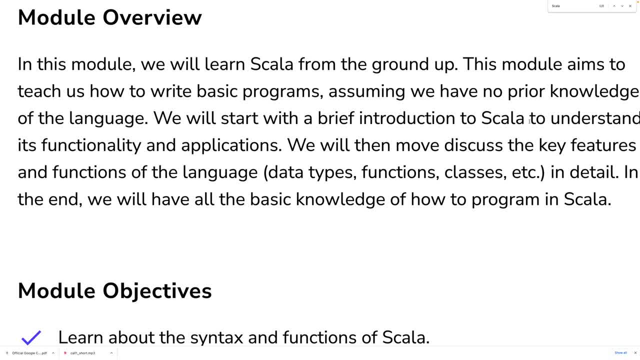 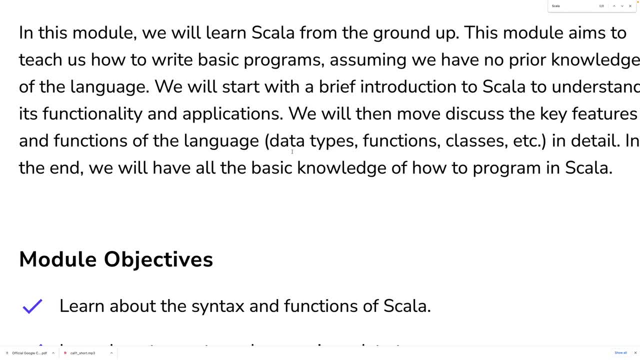 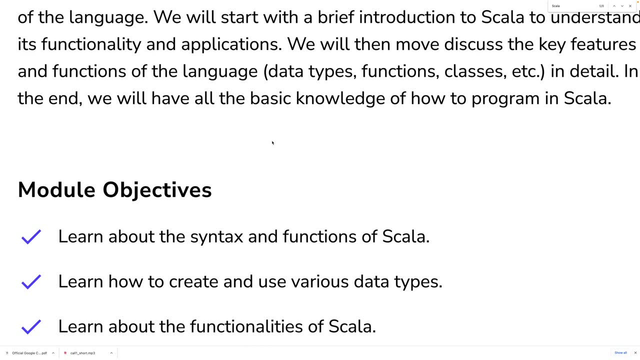 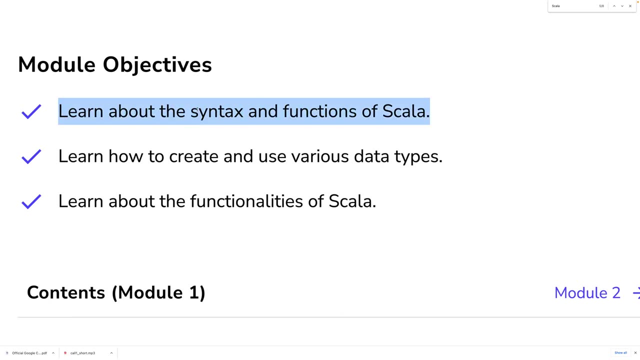 any programming language. so I will start with the brief of introduction of Scala to understand functionality and application and also I will teach more, discuss the key feature and function of language, data type, function and classes etc. in detail and in the end we will have the basic knowledge to program in Scala. so module objective: learn about the syntax and function in Scala. 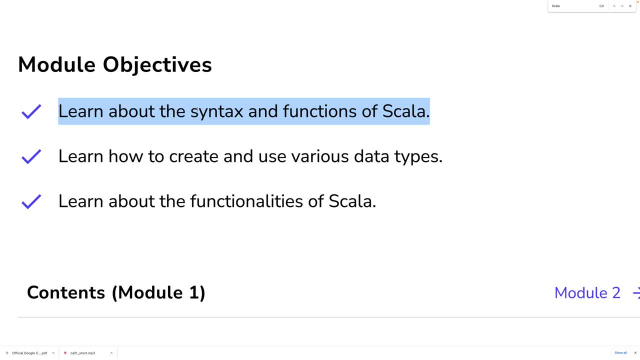 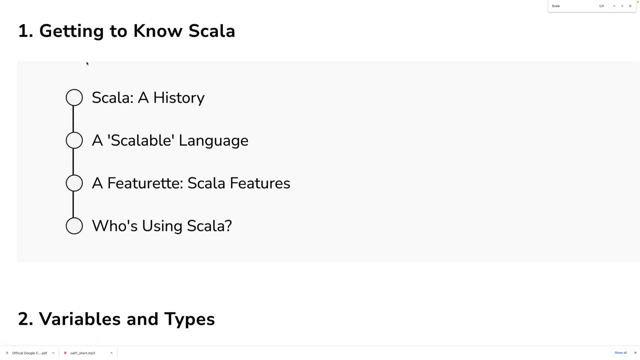 so for data engineers who want to give the interview for data engineering or who want to focus or scale up their knowledge, learn about the use variables, learn about the function and Scala. so first chapter I'm going to start is getting started, getting to know Scala and its history. 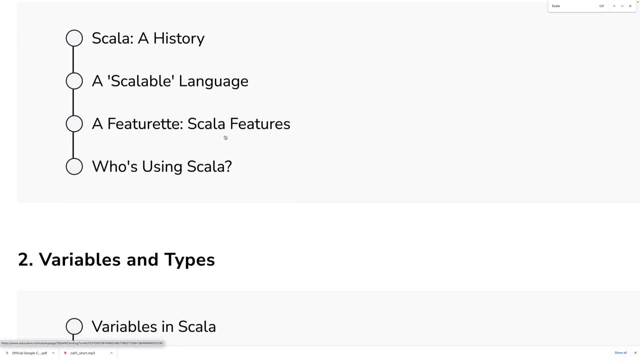 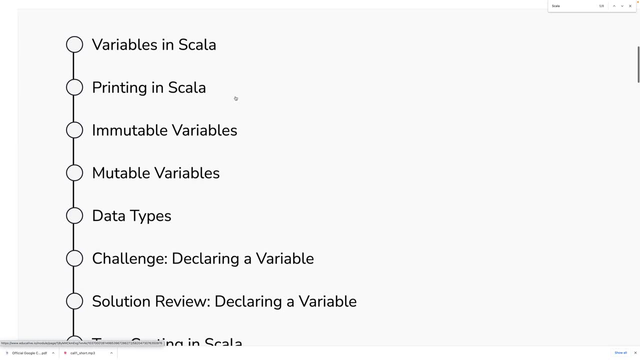 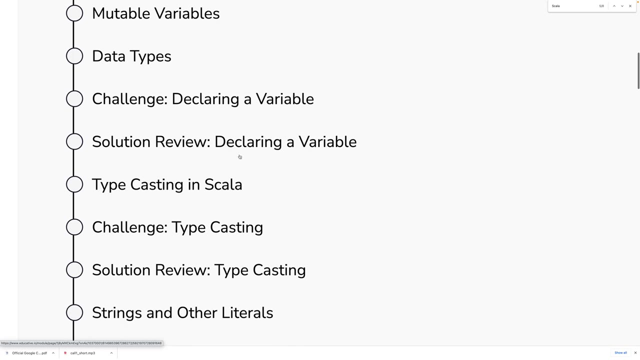 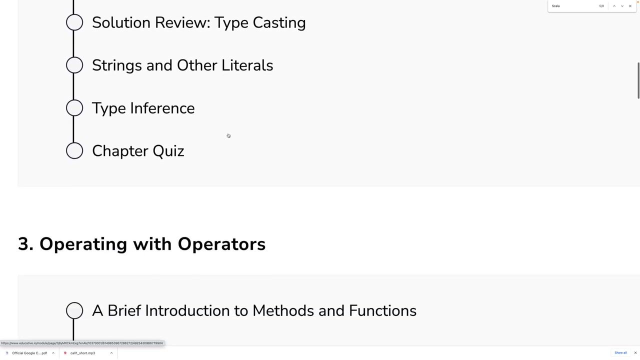 scalable language and scalar features. who are using Scala? and the next part I'm going to start is variable in Scala: printing in Scala immutable variable. mutable variable data type challenge, a variable solution degree. declaring variable type casting in Scala, challenging type casting solution review and string and other literals and type interface increase. next one I'm going to talk. 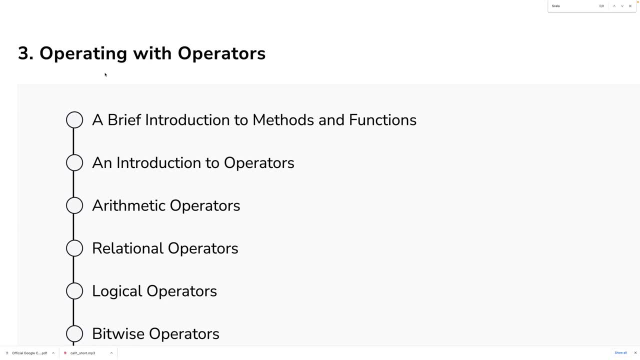 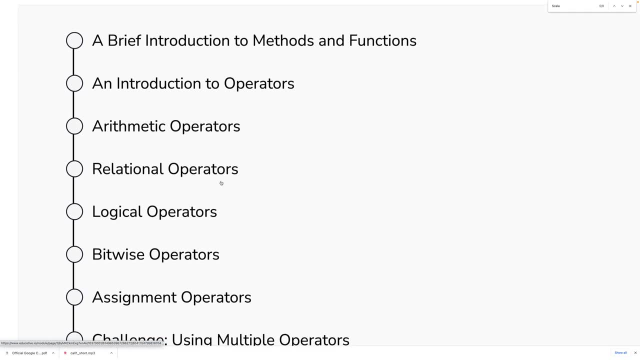 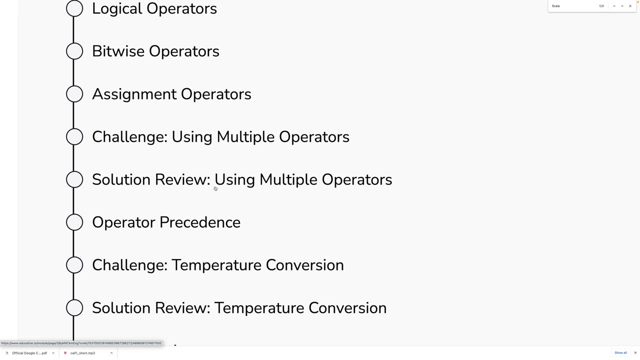 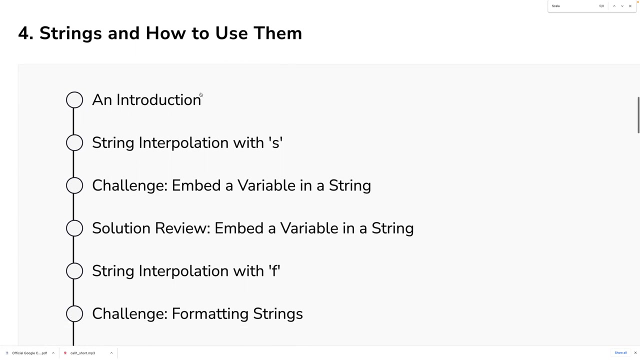 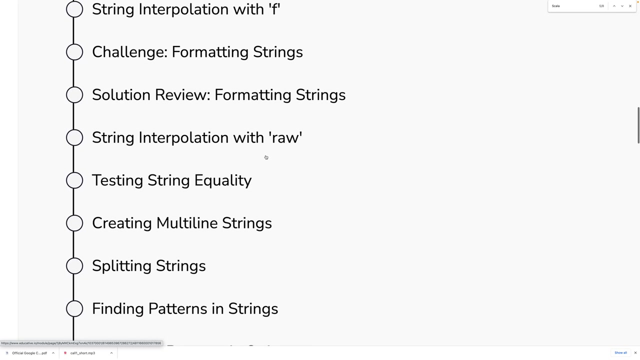 about operator and operating, so brief: introduction: method of function. introduction of operators: arithmetic operators, relational operators, logical operator, bitwise operator assignment. operator challenge using the multiple of freighter solution. operator procedure challenging solution, string and how to use them. introduction: string integration with s challenge solution. string interpretation solution review. and then we are going to talk about Scala collection library, which 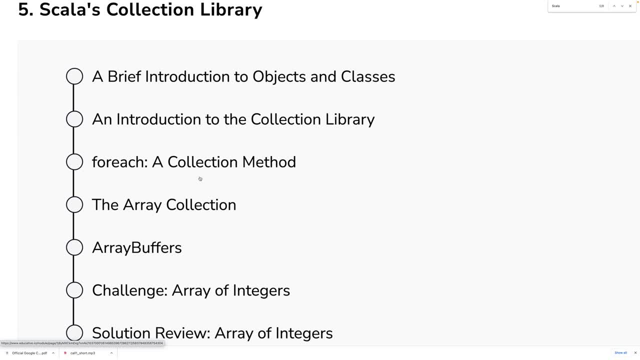 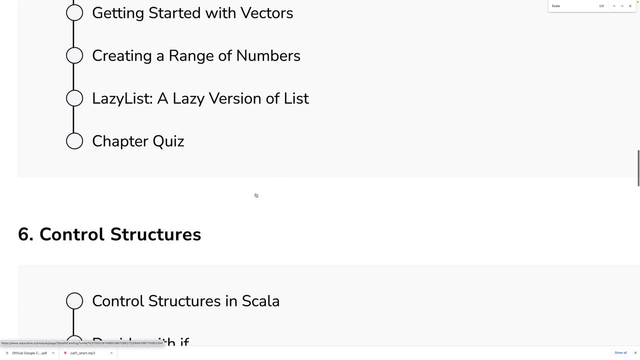 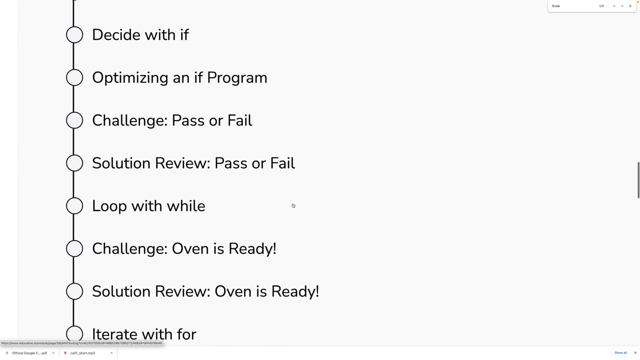 is very, very important for each, each in an array, then array buffer, then we going to do some challenging and then answer, then list and then control structure like if and as, decide if, optimize the program, challenge, pass when, solution, review and loop right. and then next part, we are going. 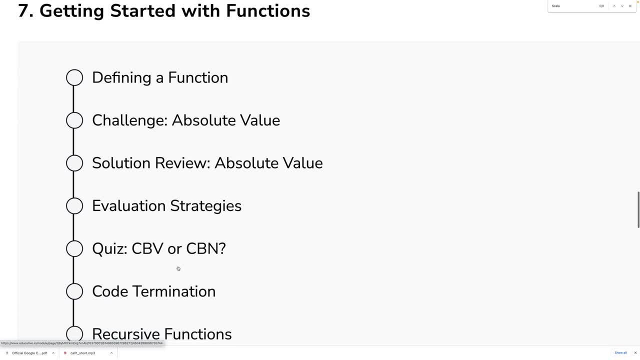 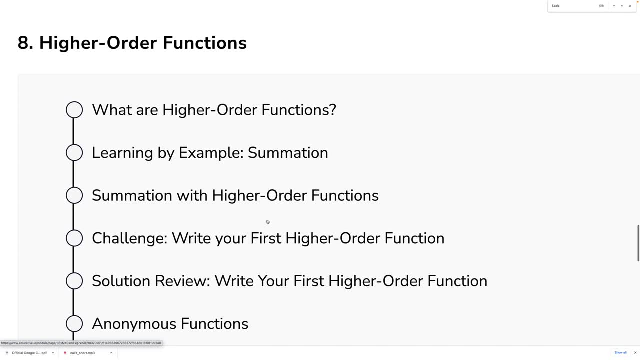 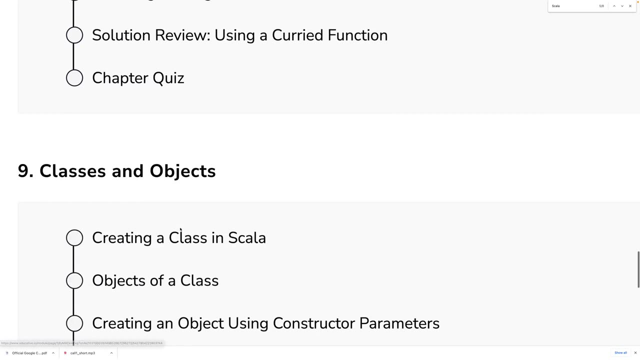 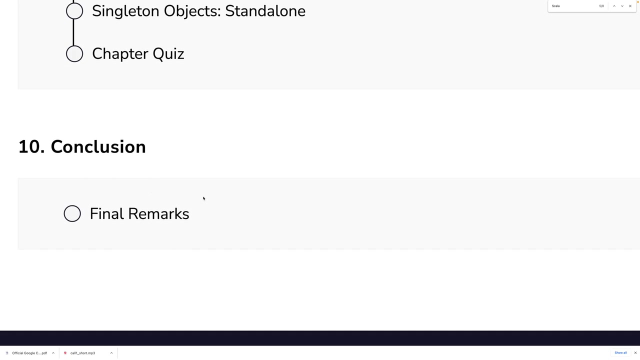 to learn about defining function, challenging, solution, evolution, and the next part is higher order function, which is also important. what is the higher order function? learning by example and simulation with the higher order function, challenging and solution. and then next ninth chapter, we are going to learn about class and abstract. and 10th final remarks. 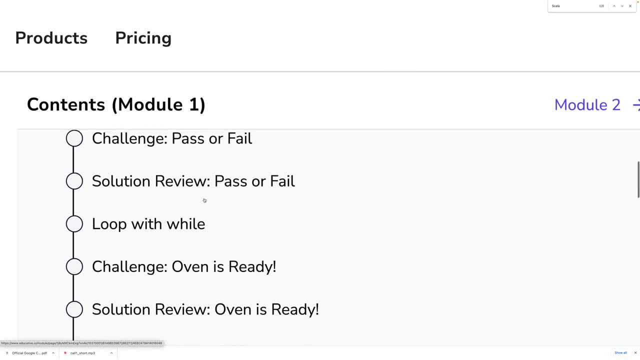 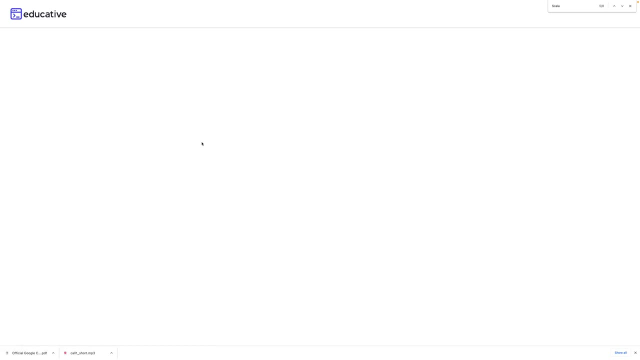 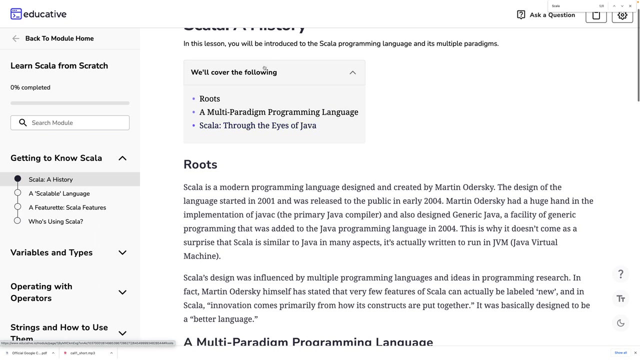 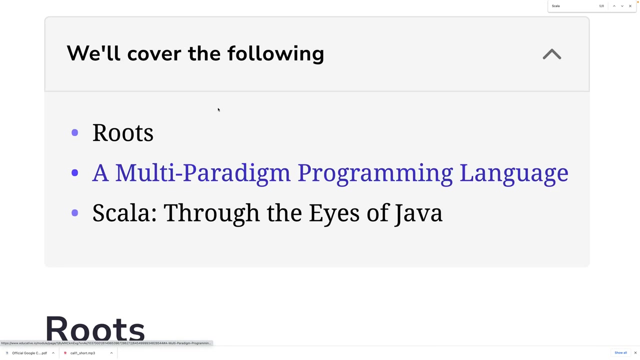 so let's go to the chapter one which is very important to learn about basic history, about Scala. let's learn about this one. so this lesson we will introduce to the Scala programming language and multiple parallelism and we will cover the root and then multi, multi parallelism programming language. then 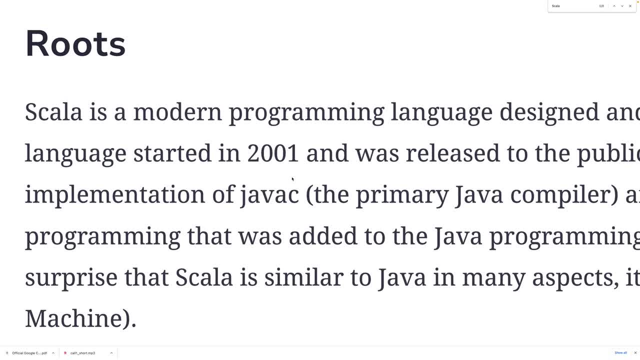 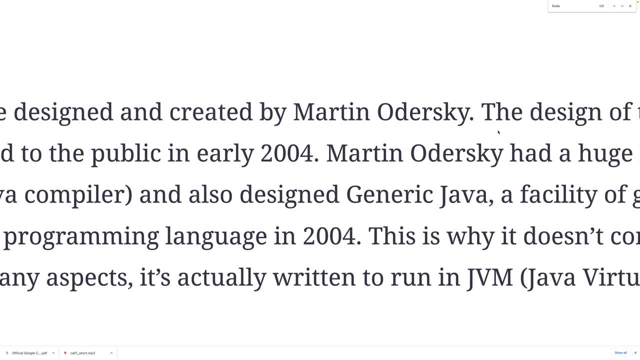 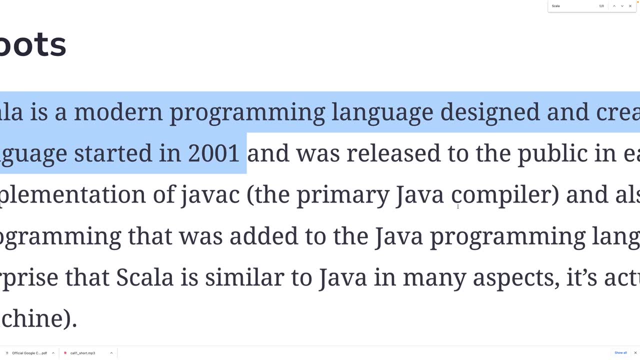 Scala through the eye of java. so Scala is a modern programming language designed and created by martin ordersky. the design of the language started in 2001 and we are going to learn about scala. so scala is in the use of the organisation system. it is founded by dr york in 2004 and the 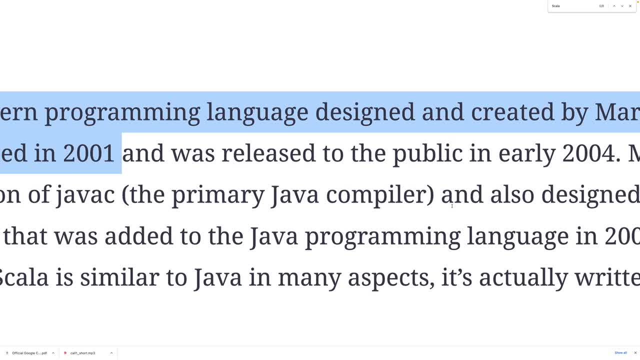 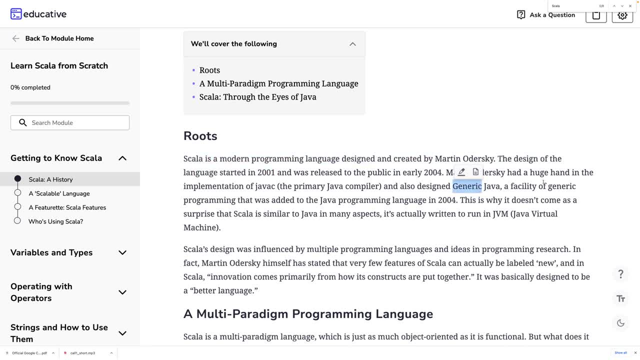 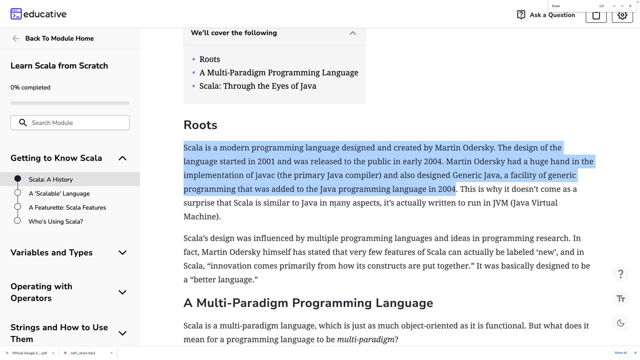 company feel honorary c press style platform and was released to the public in early 2004. martin orski had huge hands in the implementation of javac, which is primary java compiler, and also design the generic java facility for generic programming. that are in java programming, java in many aspect actually written in the running jvm java virtual machine. so scala is. 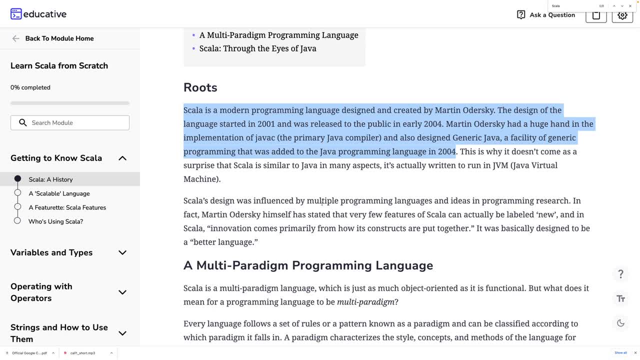 basically written in java. so scala design was influenced by multiple programming language in idea of programming research. in fact, martinowski himself has started. very few feature in scala can actually be labeled as new. in the scala, innovation comes primarily from how it's constructed and put together. it was basically designed to be the better language. the second part is multi-paradism. 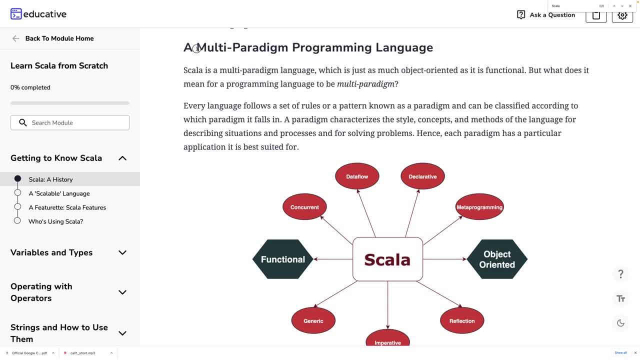 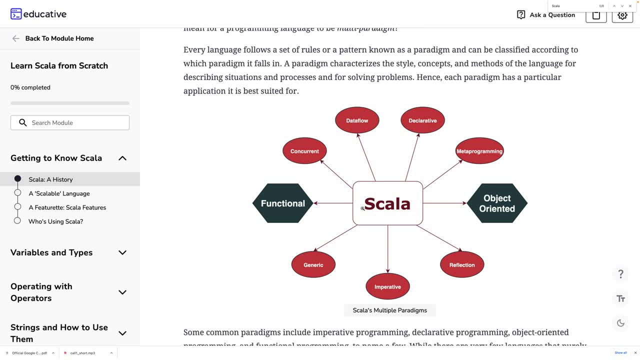 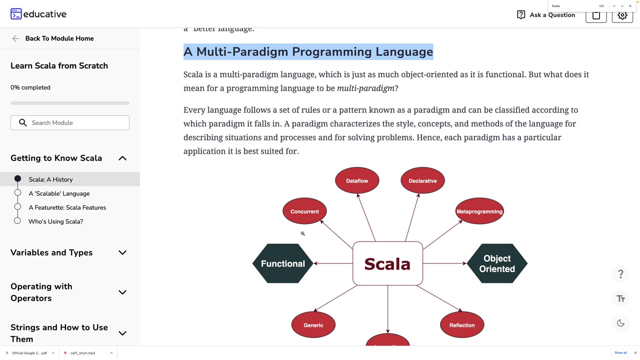 programming language. so scala is a multi-paradism programming language. so scala, generics scala, imperative scala, reflection scala, object oriented scala, meta programming scala, declarative scala, data flow scala is concurrently, scala is functional. so these two are very important. the rest are. so scala is a multi-paradism language which just as much object oriented. 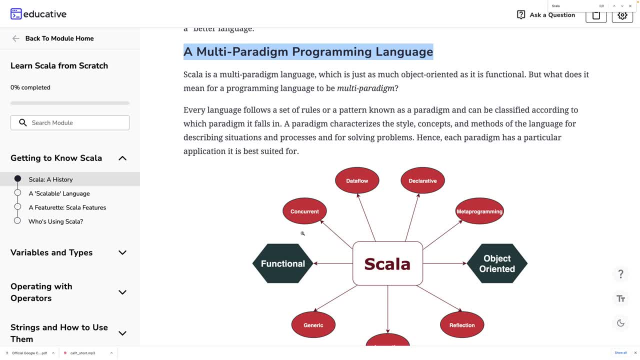 as is the functional part. what does it mean for programming? language is a multi-paradism. every language follows the set of rules and pattern to know the paradism and can classify according to the which paradism files. paradism characteristic the style, concept and method of language for a describing situation and process for a solving problem. hence each. 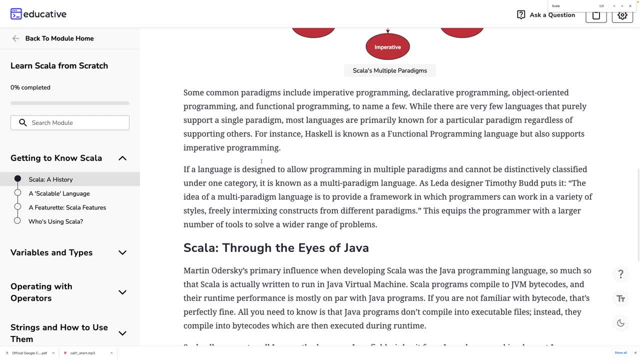 paradism has a particular application in the best sites. some of common paradism include interactive programming, declarative programming, object oriented programming, functional programming, name of you. while there are few languages purely supported single paradism, most languages are primarily known as particular paradism, regardless of supporting others. for instance, hassel is known. 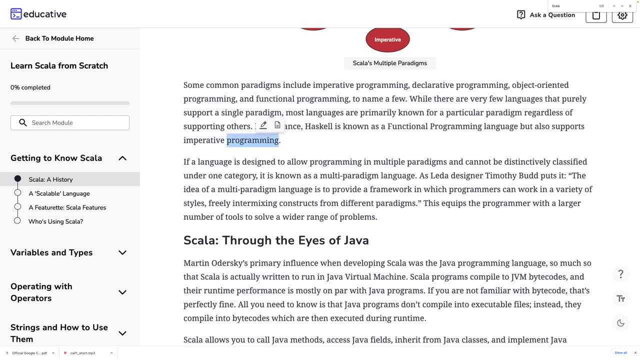 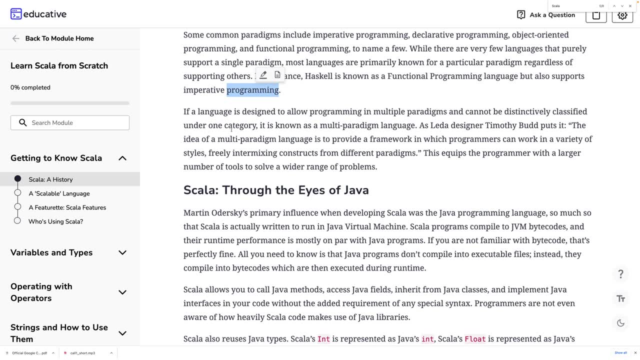 as a functional programming language, but also support imperative programming if if a language is designed to allow programming in the multiple paradism and it cannot distinctly declassified under the category is also known as a multi-paradism language. scala designed the idea of her multi-paradism. 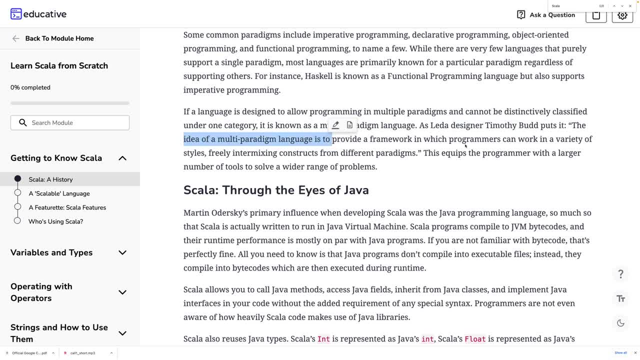 language and it cannot distinctly declassified under the category is also known as a multi-paradism language. the 20 guerrilla languages provide framework in which for a programmer can work in variety of syntax and makes things considered from different paradism. so this is a some 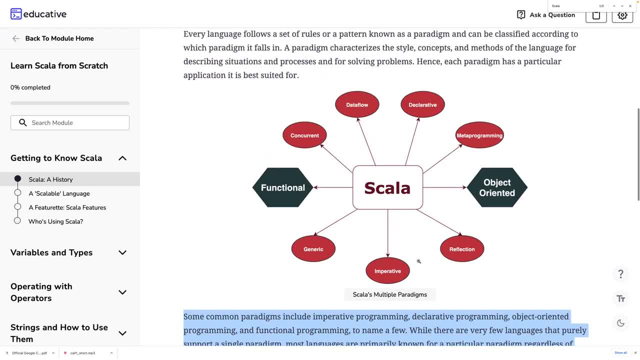 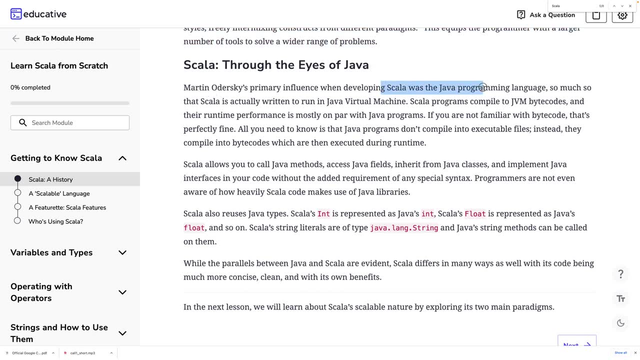 basic dream ich理 are go to talk all like is scallies. for now we're going to talk about Scala, not throw the eyes of llama. so Scala was at the Sama programming language. so that is college, actually written and running Java, virtual machine, Scala bumba- peripheral understanding. 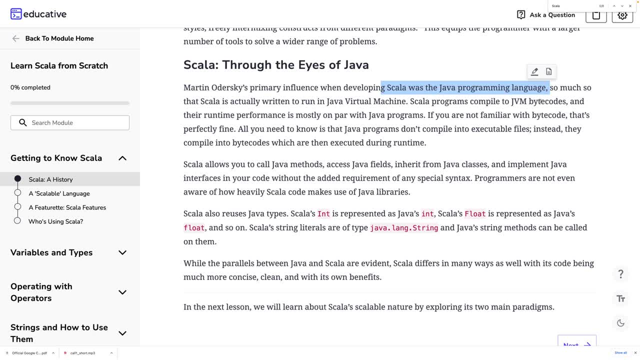 issues and simple code favorite. the app Here on the right side of the screen is bumba and the object and then the. they take them into the very within the class at which the scripting program come file to xavium bytecode and their runtime performance, mostly on for java program. 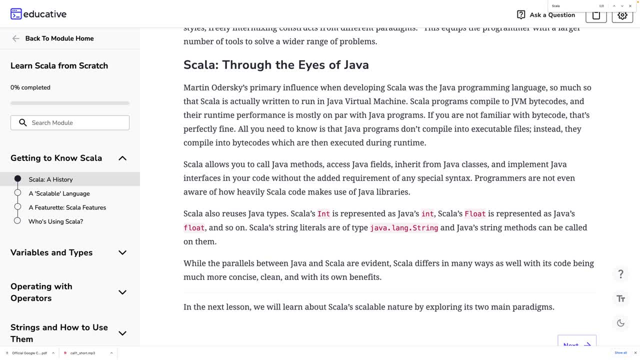 if you are not familiar with the bytecode, that's pretty fine. all you need to know that java program does just compile and execute executable file. so what we do, it will convert java into bytecode instead of they compile into bytecode, which then executed during the runtime. scala allow scala. 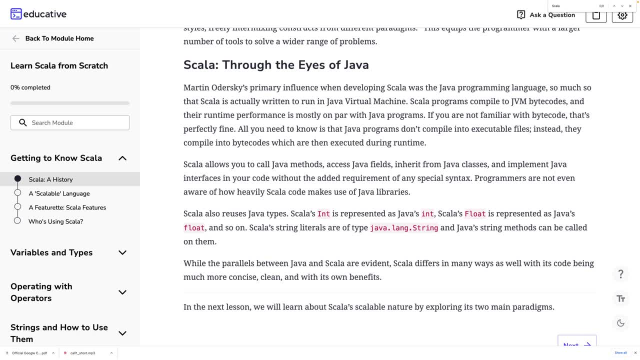 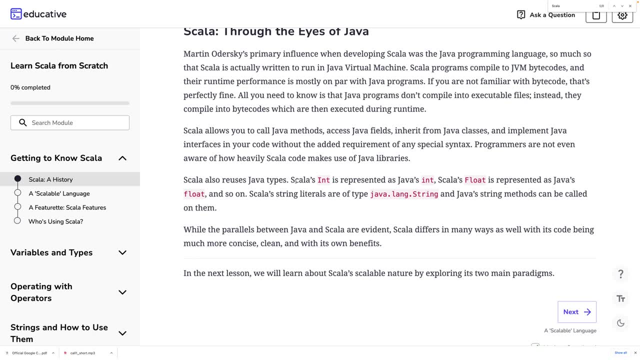 allow you to call java method access java field. in here. from java i mean scala has a. there is a way to connect this kind of scala also reuse java type. scala integer is represent java integer. scala float represent the java floats. so on the scala string literal is type of javalangstring. 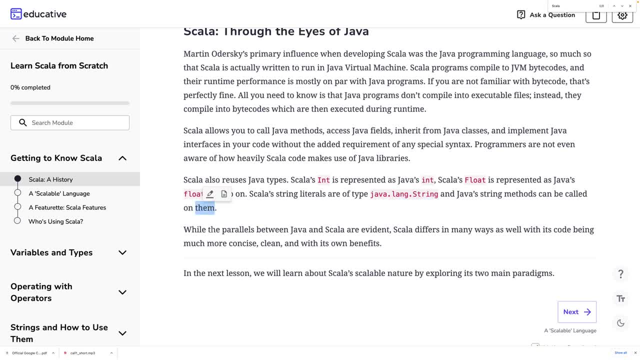 java string method can be called from them, while the while the parallel between java and scala is evidence, scala differ for many way as well, as it's a wing much and more concise and clean, with all benefit in this. in the next lecture, we will learn about the scala scalable nature by exploring two main paradigms. 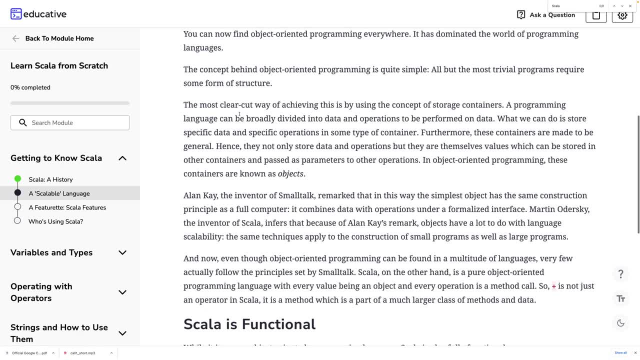 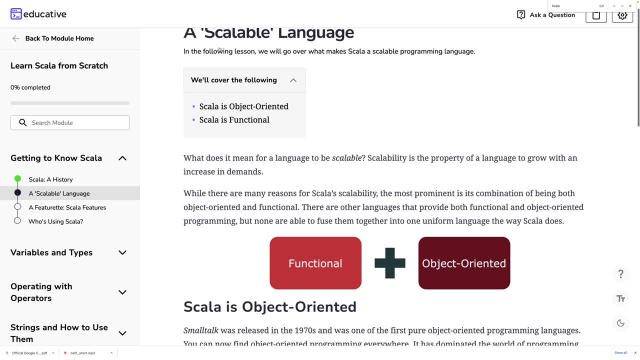 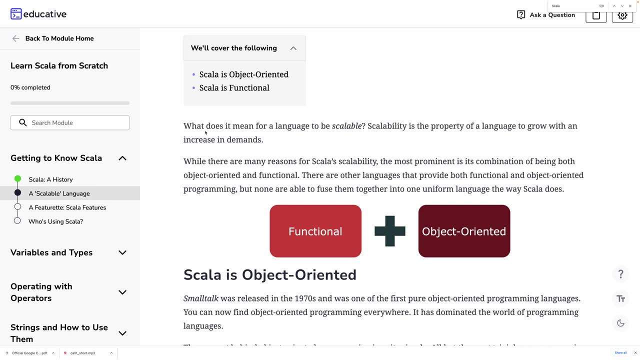 so let's go to the next part. so next part is: uh, functional plus object oriented function. scala is a functional programming and object oriented, so let's. so we are going to cover here scala, object oriented scala, functional. so these two values, object and function. so what does it mean for a language to be scalable? scalability is a property of a. 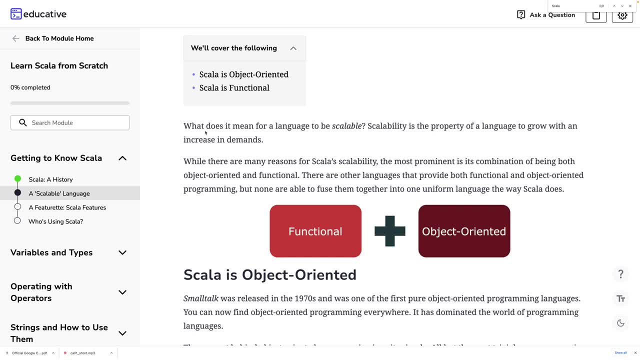 scala language to grow with and increase, increase in a demo. scalable means it, if it is scalable, so many people will use. while there are many reasons, the scalized scalability, most prominent combination is being both object oriented and function. there are other languages that provide both functional and object oriented, but none of able to fuse them together into a unique function. so we will learn. 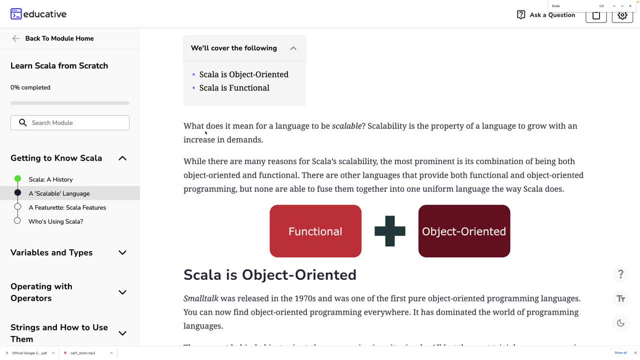 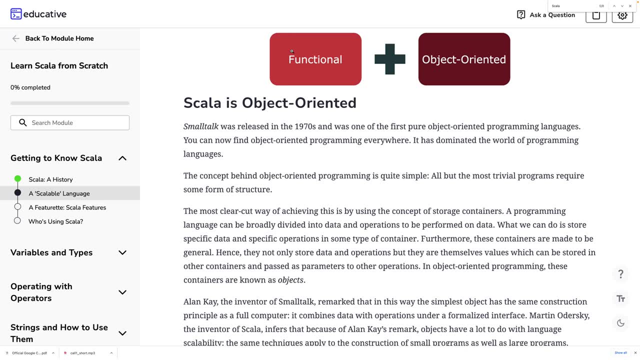 about the scala, scalability and function. so let's go to the next part. so let's go to the next part. so so i am going to introduce you with the infweitcps project. this project involves different types of object oriented programming and we are going to introduce you guys in the next. 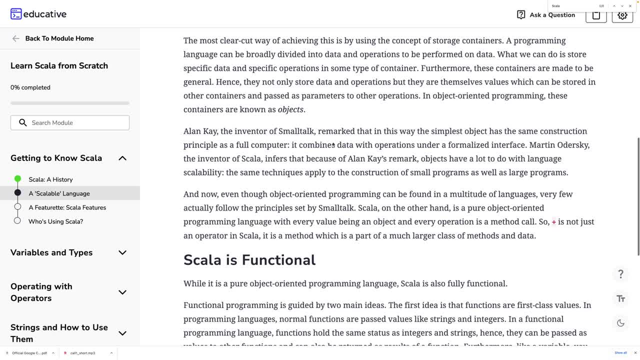 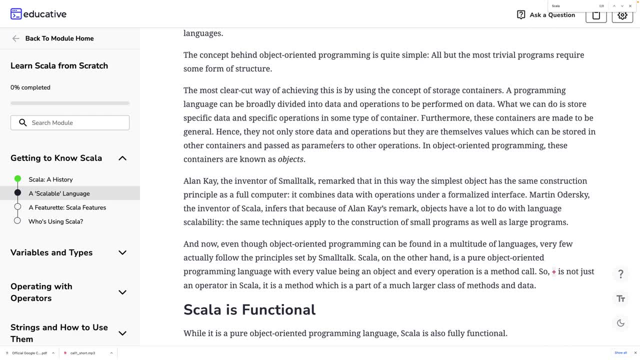 some form of structure. so most clear-cut way to achieving this by using concept, was stored a container. a programming language can be broadly divided into data and operator to be performed on the data. what we we can do, it is stored a specific data and specific operator on the some type of 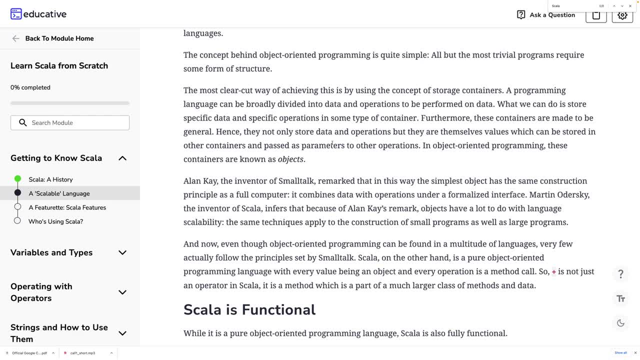 container. furthermore, these container are made by general, hence they are not only stored data and operation but also themselves values which can be stored in another container. pass as a parameter: other container, object oriented programming. these container are known as object. so object. this is definition of object. Ellen key is a inventor of a small talk. remark that in this ways, 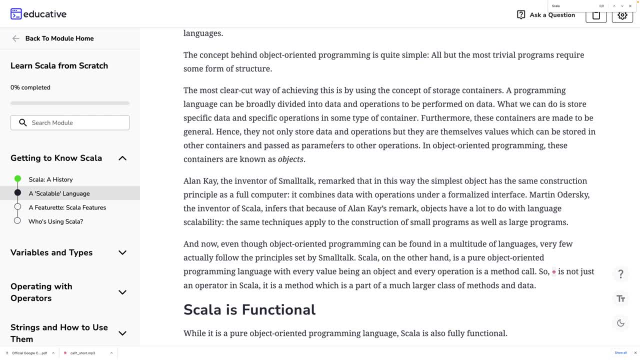 simplest objects has the same construction principle and full computer. it combines data with the operator under the formalized interface. Martin orders, key inventor, the Scala interfere. become a Ellen key reminder object. have a lot of guru language scalability in the same technique apply to the construction of a small program as well as large program and now even. 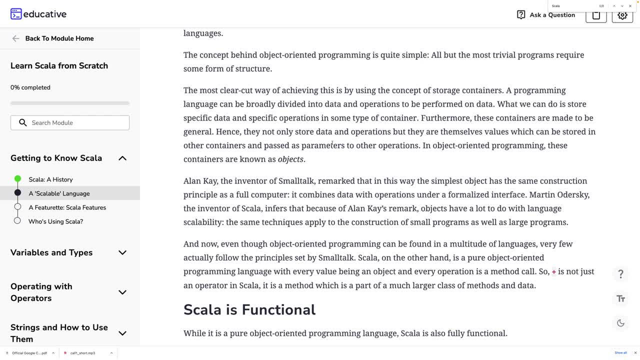 though object oriented programming can be found in multiple language, very few actually follow the principle set by small talk, small talk. Scala is, on the other hand, and in pure object oriented programming, language, with every value being is object and every operator method is called. so plus is not just a. 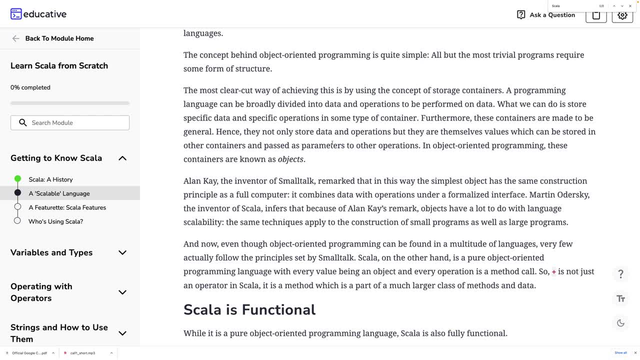 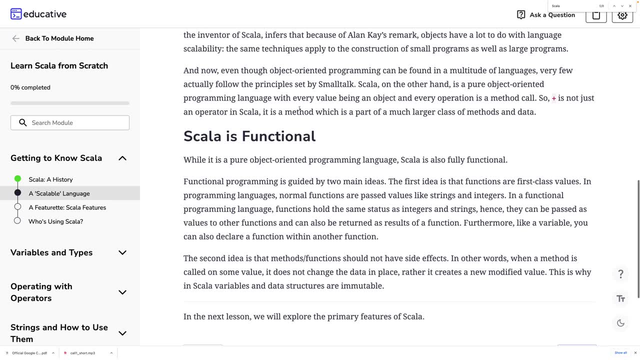 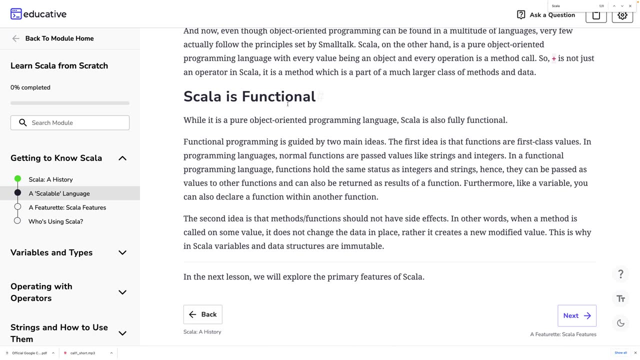 operator from in Scala, what is a method which a part of much larger class method of data. so this is the which we learn about. you know the object. paradise them now we are talking about to Scala functional. well, it's pure object oriented programming language. this color is a fully functional. 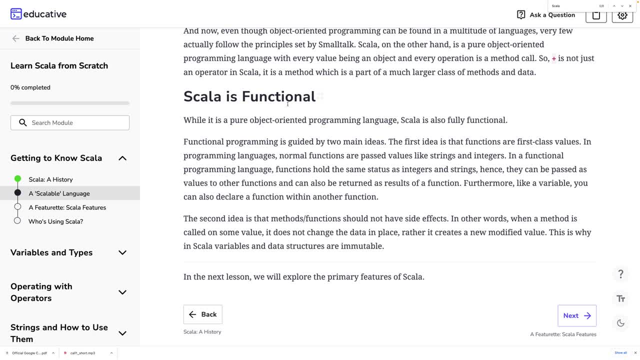 functional programming is a guide by two main ideas. first idea is the functional, our first class value in the programming language, normal function, our past, ok, a Values like string and integer in the functional programming language function hold the same status as an integer and a string. Hence they can be passed as a values, other function and can also be written the result of function. 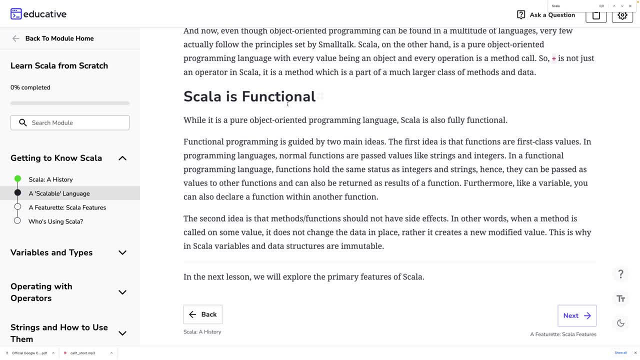 So, furthermore, like variable, you can declare in the function within another function. so the Scala Idea is that method of function should not have a side effect. In other words, when method is called, some value does not change the data place rather than create a new Modifies value. This is why Scala variable and data structure are immutable. 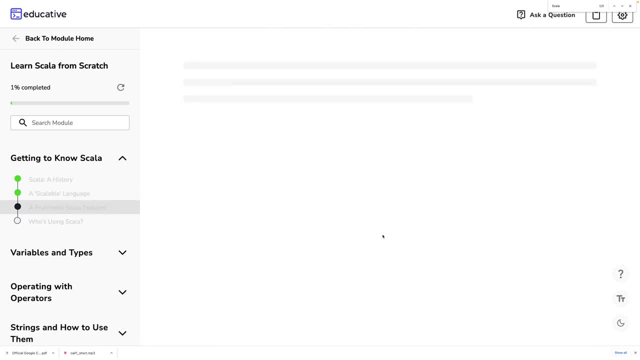 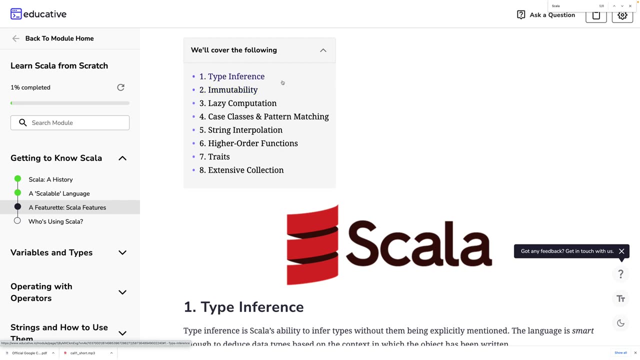 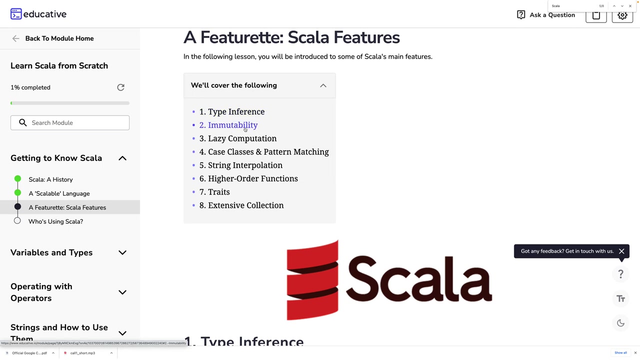 Okay, so these are relation we are, we learn and Features of Scala. so now we talk about the some feature basic feature about is Scala. So This feature I'm going to talk type of interface: immutably D means it cannot change a lazy computation which is also used in a spark in later the chapter, case class and pattern matching. 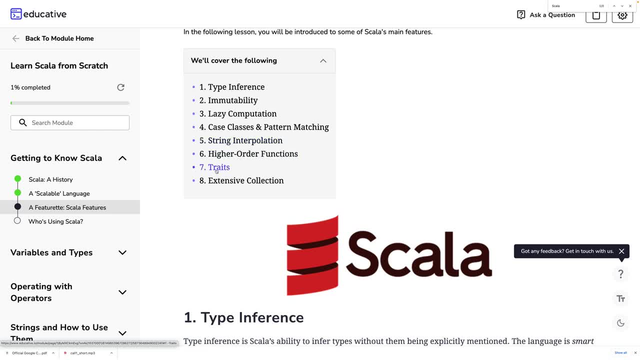 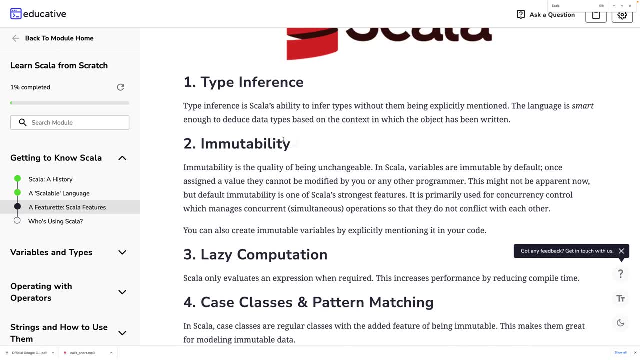 string interpolation, higher order function and traits and Extensive collection. So these are very important type of interface. So a type of interface in Scala, ability to Infer type without being them explicitly mentioned. the language is a smart exclude, detect data type based on the context which you observe it in in 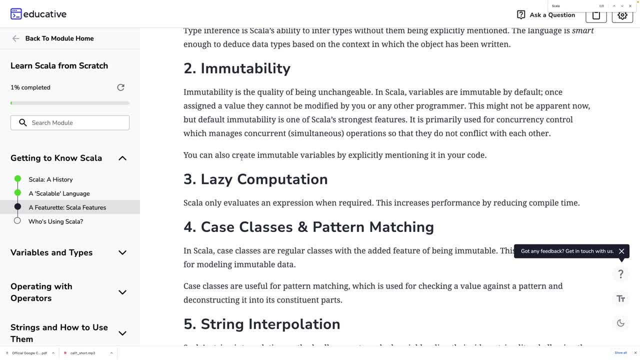 immutability. immutability- Quality being- is unchangeable in a Scala variable- are Immutable by default once assigned to value 2. cannot be modified by you and you are the programmer. This might not be Apprent now, but default immutably. one of the Scala strongest feature. It's a primary use for concurrency control, which 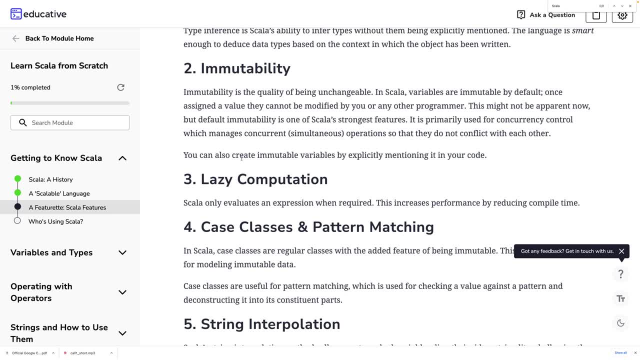 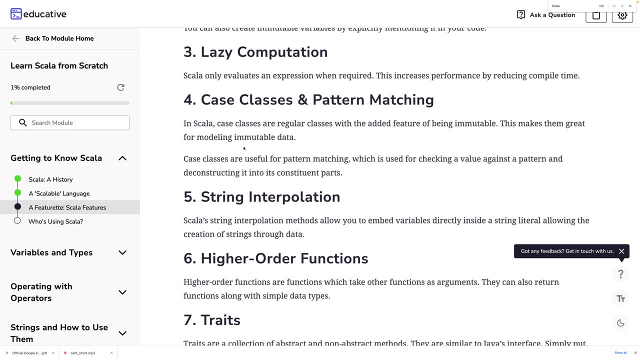 Manage the concurrent Operation that do the conflict with each other. you can also create immutable variable by explicitly Answering in your code. Next part is very important: lazy Computation or evolution, so Scala only will it an expression when it's required. This is increase the performance by reducing compile time, case class and pattern matching in. 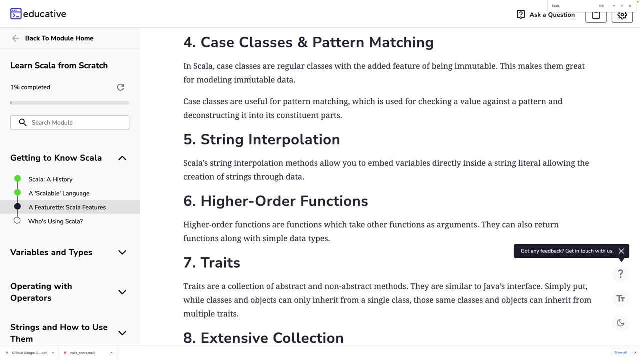 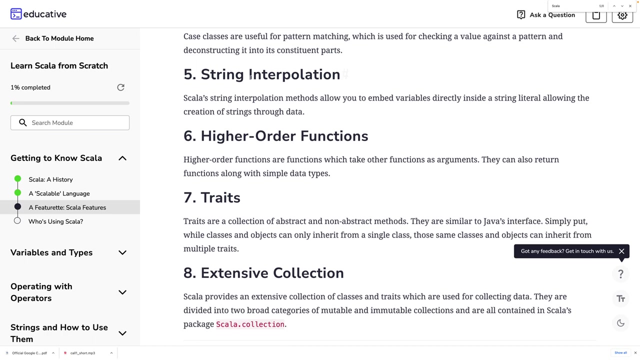 Scala case class are regular classes with the added feature being the immutable. This makes them a great modeling. immutable data case classes are useful for pattern matching, Which is used for Checking the value against pattern and deconstructing into the constant pattern string interpolation. so string interpolation method, allow you to